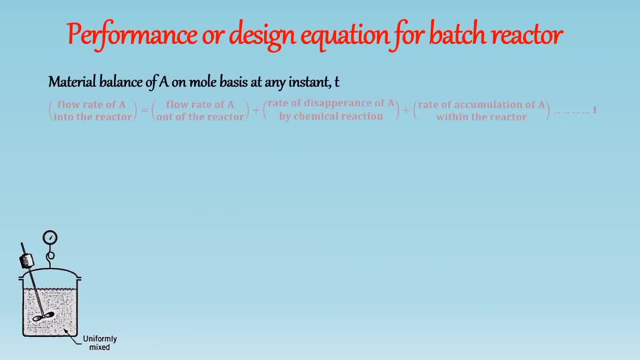 time t. So we get: flow rate of A into the reactor is equal to the flow rate of A out of the reactor, plus rate of disappearance of bichemical reaction plus rate of accumulation of A within the reactor. Equation number 1.. 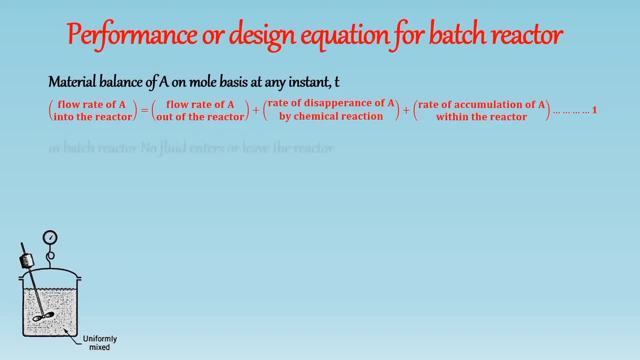 So, as we know, In batch reactor No fluid enters or leaves the reactor during the course of the reaction. Hence the flow rate of A into the reactor and The flow rate of A out of the reactor is equal to 0.. 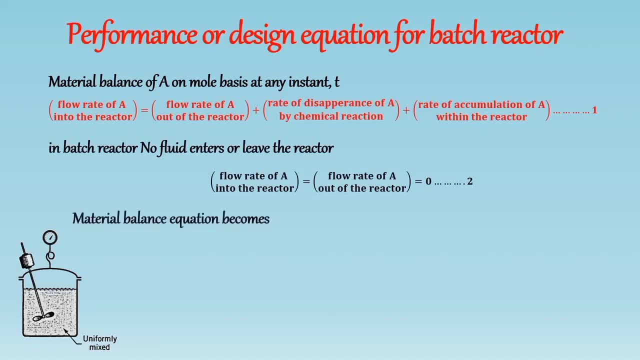 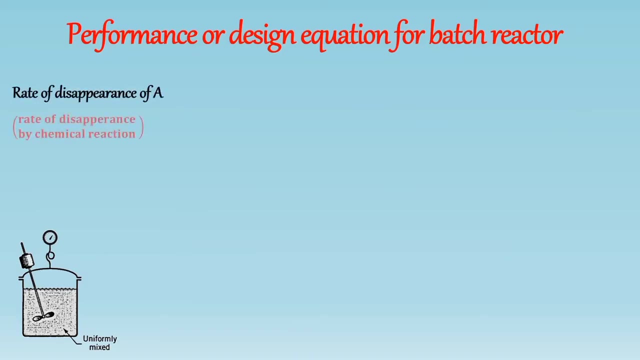 Equation number 2.. And material balance equation can be written as Now: let's calculate the rate of disappearance of A by bichemical reaction. So rate of disappearance of A by bichemical reaction, reaction in moles per unit time in reaction volume V is equal to minus R a. 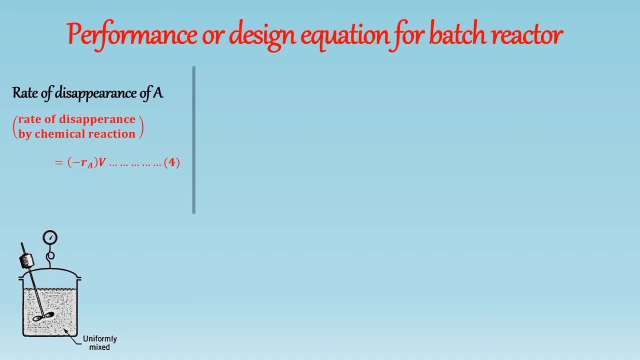 into V. now let's calculate rate of accumulation of egg within the reactor. so rate of accumulation of egg within the reactor in moles per unit time is equal to DNA by DT. but, as we know, n a is equal to moles of egg remained at T. 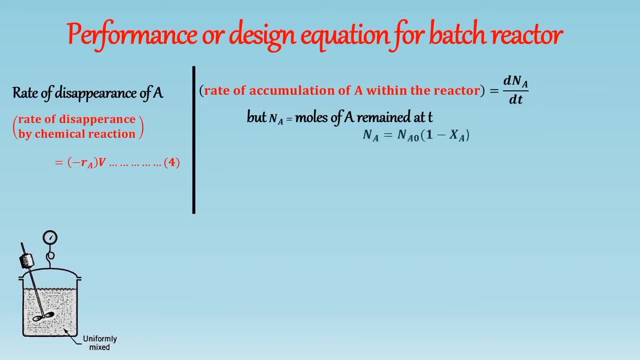 which can be written as: n a is equal to n a 0 into 1 minus X a. hence the rate of accumulation can be written as: after solving it, we get so after putting the rate of disappearance in rate of accumulation in equation number three. we get so after rearranging the terms we get now: 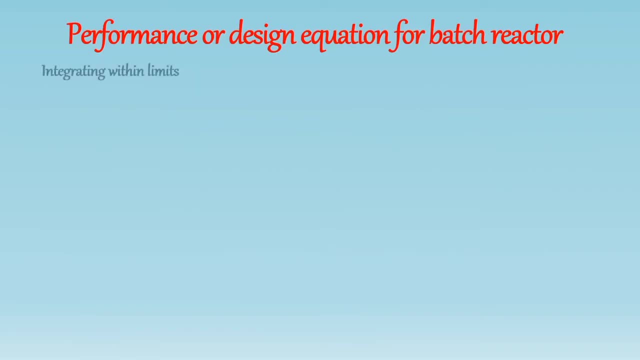 let's integrate this equation within the limit: at T is equal to 0, X a is equal to 0 and at T is equal to T, X a is equal to X a, so we get. hence this equation is a general equation showing the time needed to achieve conversion. this equation, also called as general design or performance.